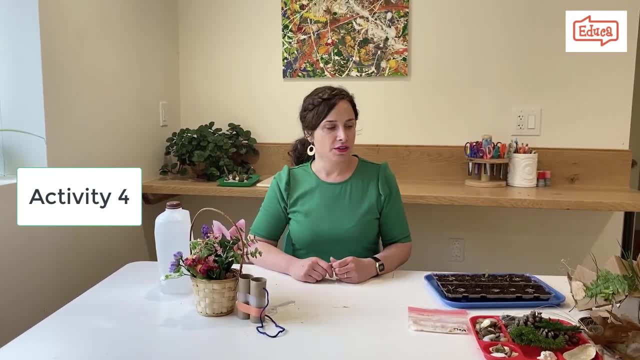 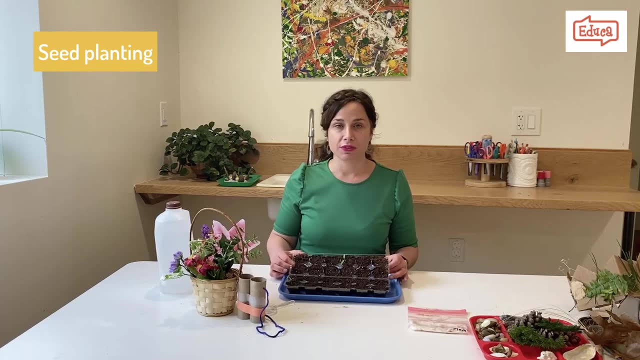 It's not always easy getting kids to connect with nature, so today I thought I'd go over a few different activities that you can do from your own home. One activity is to get kids planting seeds and watching them grow. I've used an empty egg carton for this. If you don't have a kid-sized 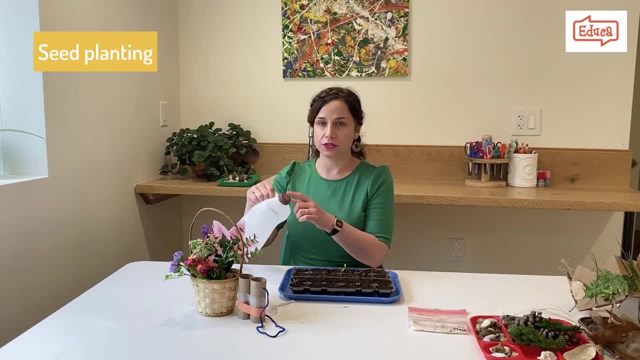 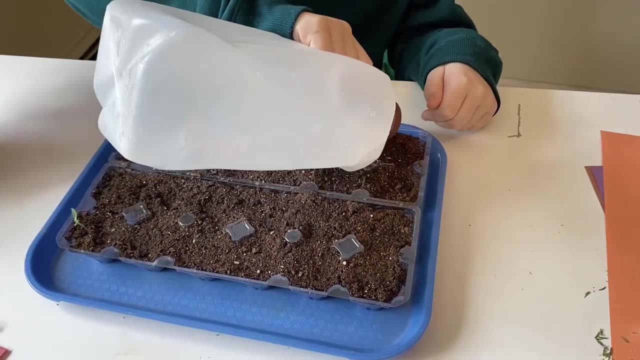 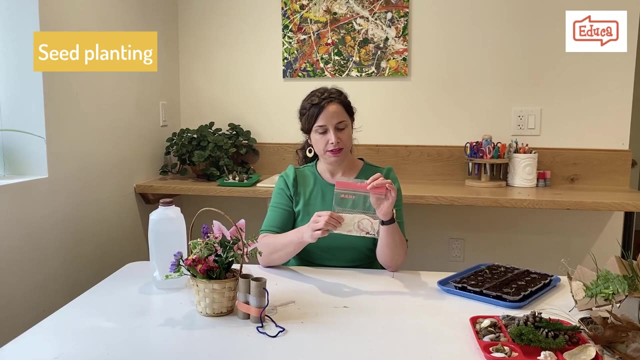 watering can. you might consider using an empty milk jug and poking some holes in the top. This particular shape is really great for young children and it's also really light and easy for them to use. Another way to watch a seed grow is to take a bean and put it behind a wet napkin or 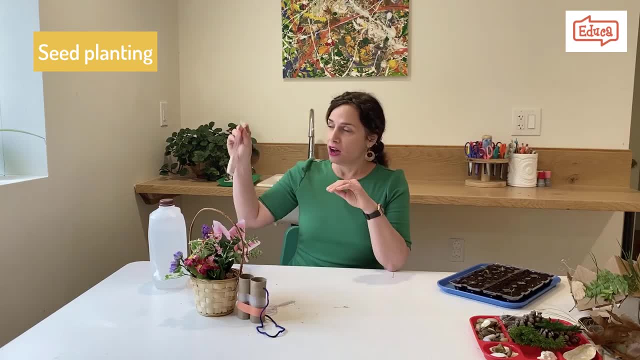 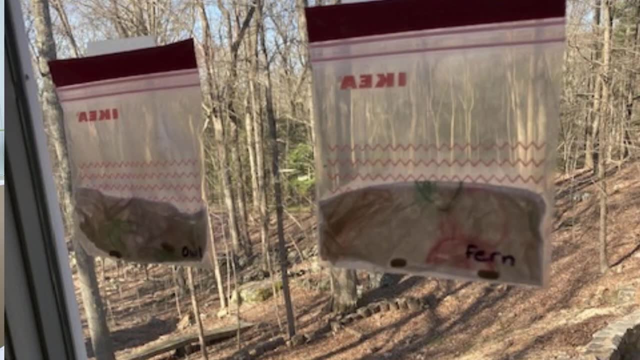 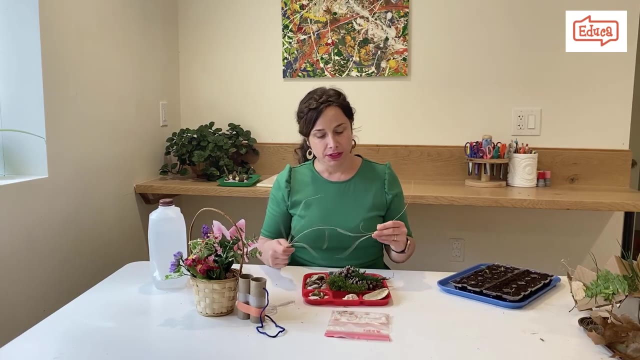 paper towel inside a plastic bag and then hang that bag on a window. You can then watch that seed grow, and it's really a neat way to have children be a part of this bean sprout life cycle. I'm always a big fan of bringing nature home into your home and using it as a building material or 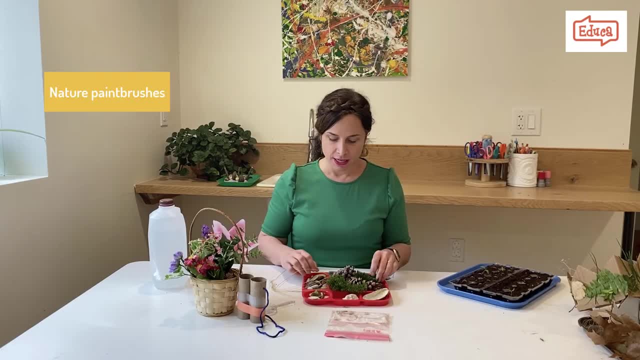 mark making material. I've been a big fan of bringing nature home and using it as a building material or mark making material for their home. I've been a big fan of bringing nature home material. these can become paint brushes when attached to a stick and if your child is playing. 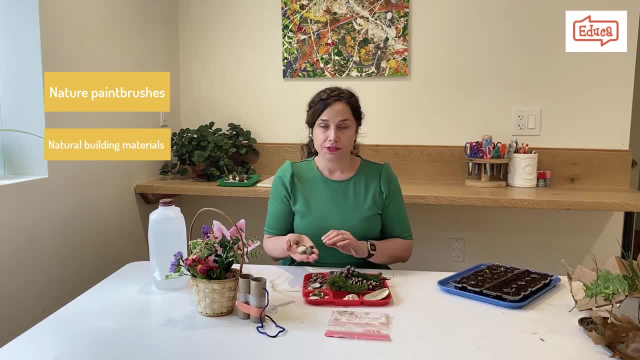 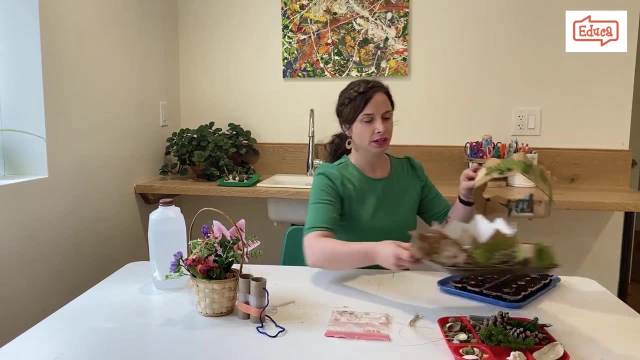 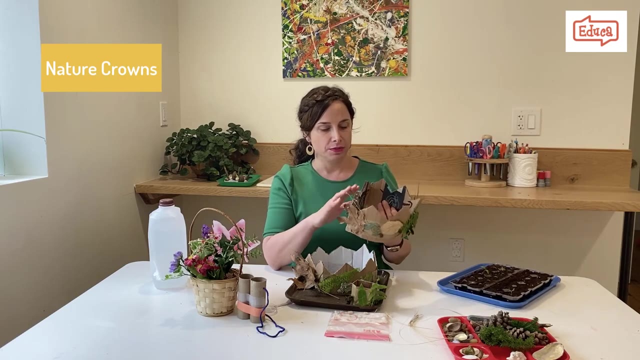 with blocks or another building material. it's great to introduce some natural materials into the mix. if you have access to the outdoors, either in your backyard or a park, you might consider making a nature crown. this nature crown is made from cardboard and then some sticky tape that 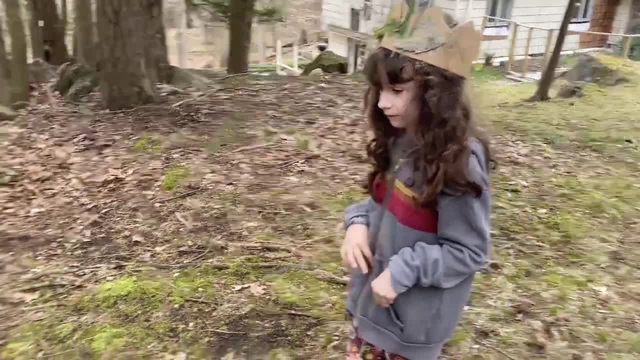 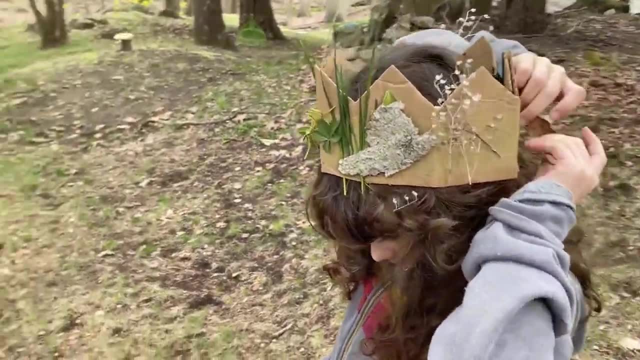 i've just stapled on, but you can also use a double-sided tape. so i've given these to my children and they walked around and collected different aspects of nature and then they bring it home and they can discuss it. these are a spring nature crown, but you can certainly make them in. 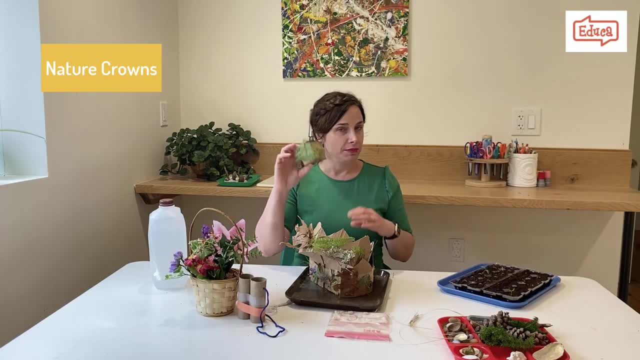 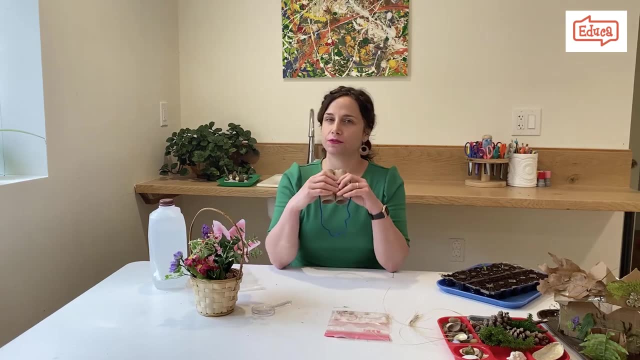 different um seasons as well. if you don't want to make a crown, you can make a cuff or a belt again if you are outdoors. one way to get kids to focus on a specific aspect of nature is to give them these kid binoculars where they can look through and really describe what they're. 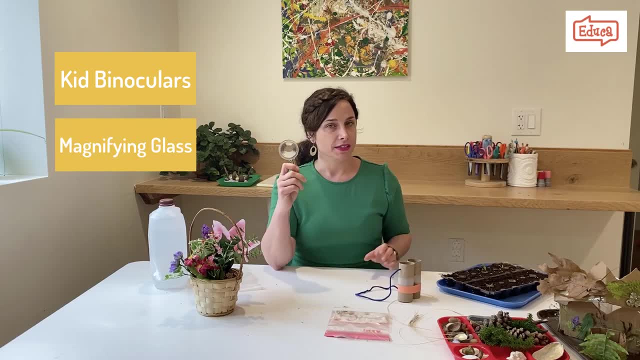 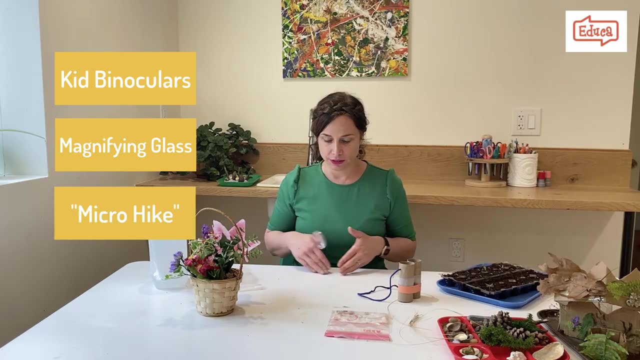 seeing in a small area. for older kids, it's great to give them a magnifying glass so they can understand nature at the tiniest level. one of my favorite activities is a micro hike, where you take one square foot of earth and you stare at it for a long time and notice. 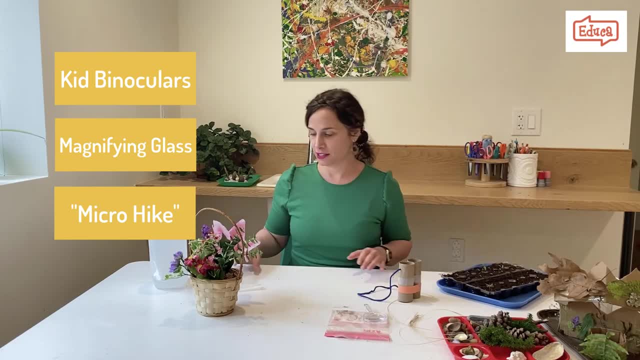 all the signs of life. it's especially fun in the spring, when there's lots of insects being born. you can also take home a little bit of nature from your park or backyard and put it between two pieces of wax paper and then use it as a sun catcher on a window.